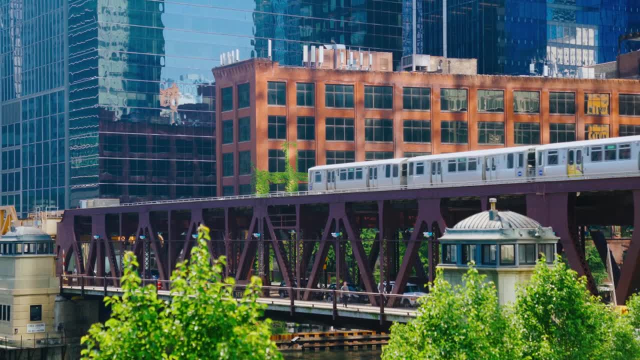 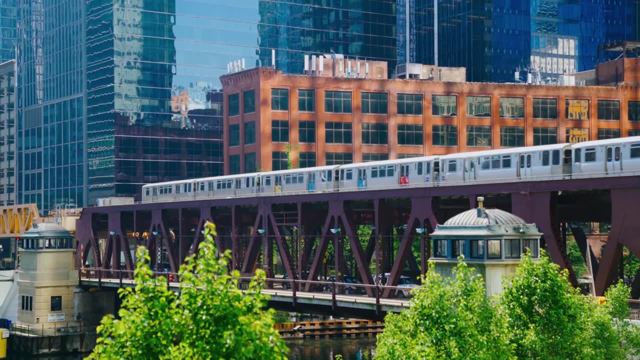 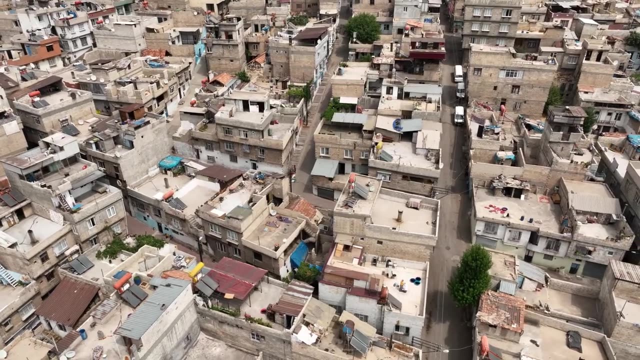 of goods and services at their disposal. High-density areas that invest in public transportation and urban planning can create a unique cultural landscape and vibrant communities that can offer more social and economic opportunities for the residents of the city, But, on the other hand, cities that have poor urban planning and lack quality public 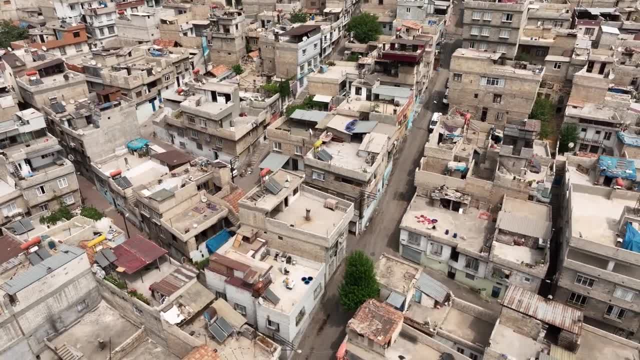 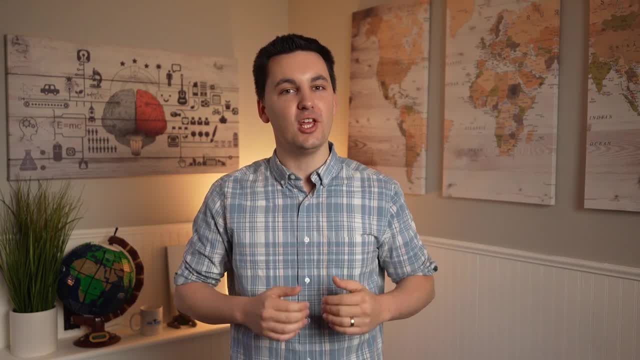 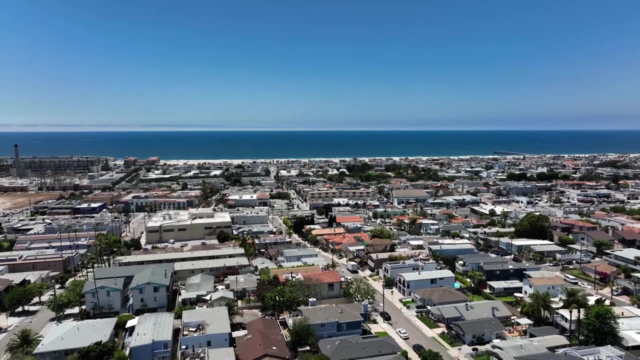 transportation and infrastructure, often see food deserts and a lack of economic and social opportunity for residents. Moving outward from high-density areas and into medium-density areas, we can see that buildings start to shrink, high-rise apartments start to shift to low-rise apartments, more multi-family and single-family homes start to appear and people 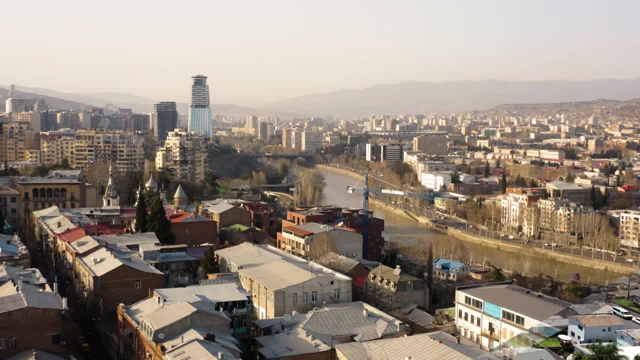 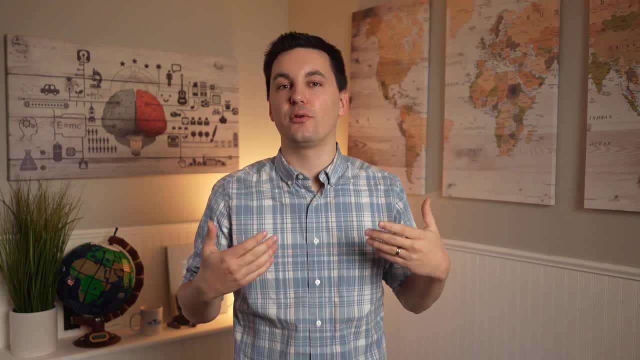 start to have room for a small front yard and backyard Now. medium-density areas are still often close to high-density areas, so they still have limited space. However, oftentimes they start to have more of a suburban feel instead of just an urban one. Restaurants and stores are. 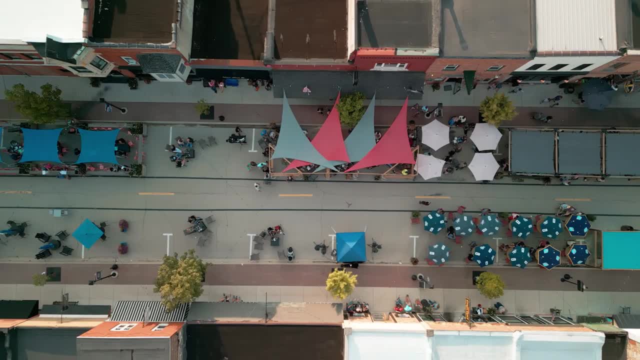 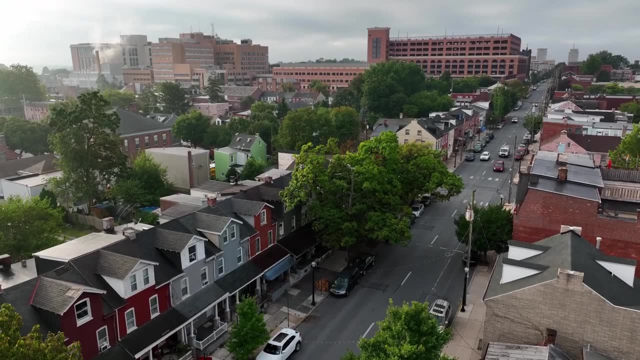 spaced out from residential homes, but still remain in close proximity to residential areas. Speaking of residential areas, we can see that they often have more diversity in the types of homes. It is common to see townhomes, duplexes, triplexes and single-family homes all in one. neighborhood. Now, as we continue to move farther away from the CBD, we will eventually get to low-density areas which have the most space available. Here, homes are often single-family homes or a few low-rise apartment buildings. The average lot size is much larger compared to the 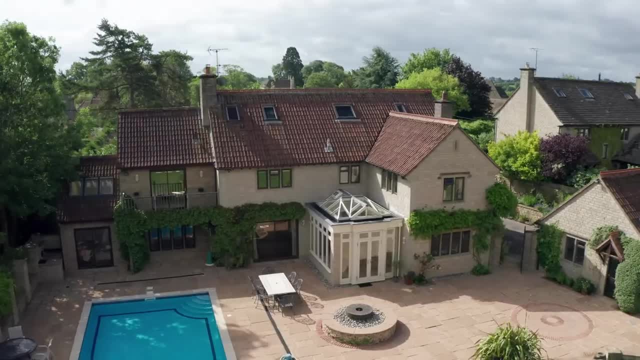 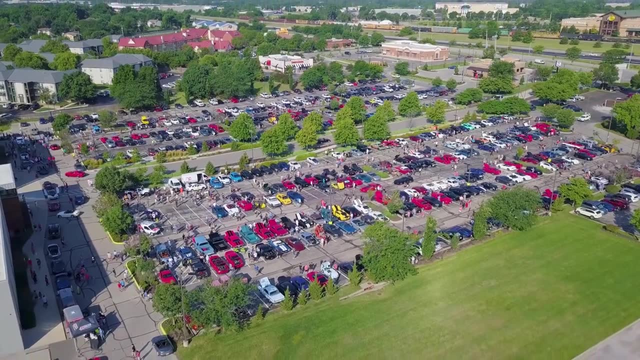 lot size in a high-density area, allowing for more buildings to build outwards horizontally instead of having to build upward. There's also more green spaces in low-density areas, room for parking lots and larger roadways, all of which allows residents to not only get around. to the local area, but also allows them to get in and out of the larger urban area. Generally, low-density areas require more land for the same number of residents as high-density areas, which leads to increased commute times and a larger dependence on personal vehicles to get. 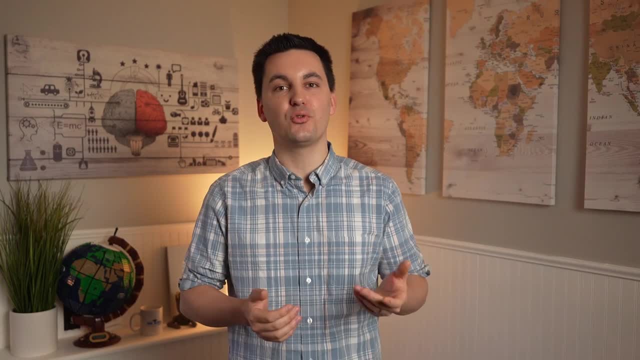 around. In addition, low-density areas require more land for the same number of residents as high-density areas, which leads to increased commute times and a larger dependence on personal vehicles to get around. These areas often lack public transportation, as it's uncommon for those. 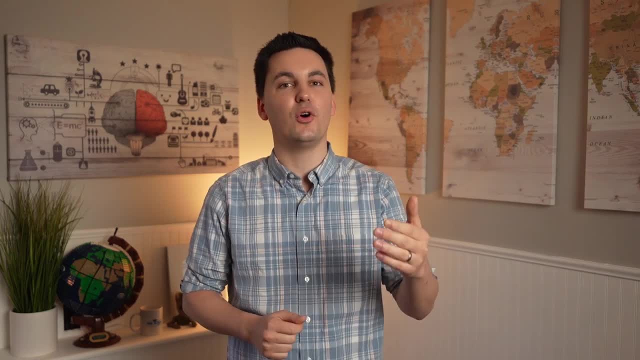 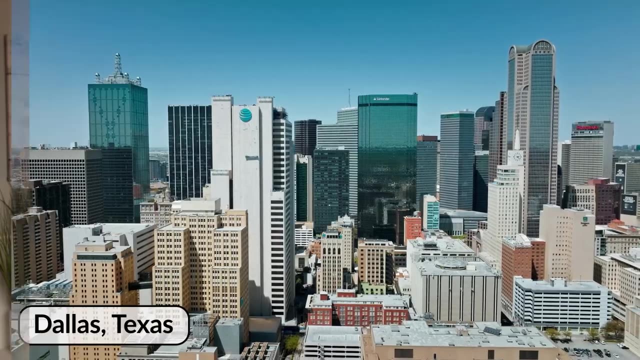 services that exist in high-density areas to extend this far away from the CBD, putting a larger reliance on automobiles for travel. Now, of course, all of this depends on where in the world you are looking at. For example, while large skyscrapers are more common in large urban areas, 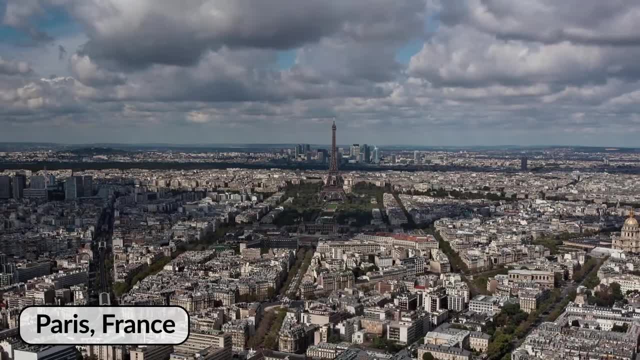 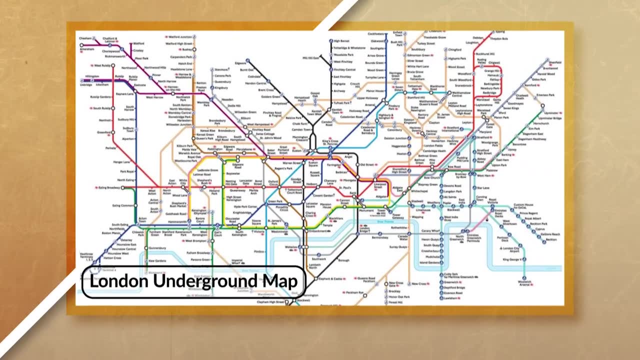 in the United States. the same is not true for all European cities. Oftentimes we see cities that put height restrictions on buildings to create a specific city landscape. We can also see that many European cities often tend to have more public spaces, and that's because they're